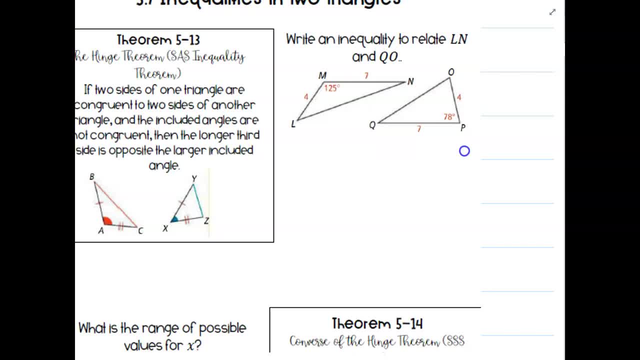 with a form. so for this first one, if we want to write an inequality to show the relationship between L in and Q, okay, now look at what we have here. we have two congruent sites: this ML measures for and QP measures for. so those are congruent if in measures 7 and QP measures 7. so notice that I have these. 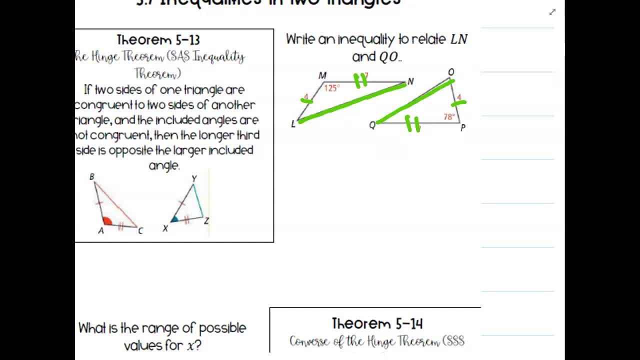 two sets of congruent sites and they give me the included angle. now it has to be the included angle, being all in between. okay, but notice, angle M is 125 and angle P is 78. this is the angle that we want to write, and this is the angle that we want to write. 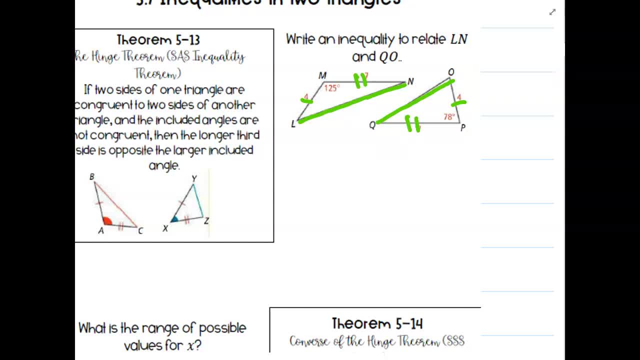 this is the angle that we want to write. this is the angle that we want to write. this is the bigger angle. okay, since angle M is bigger, what I can conclude? since the sides that are created are congruent, I can conclude that L? in is going to be greater than QO, since the sides are congruent. that's the big thing. 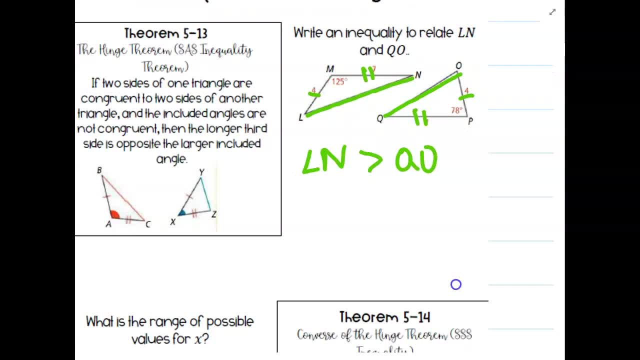 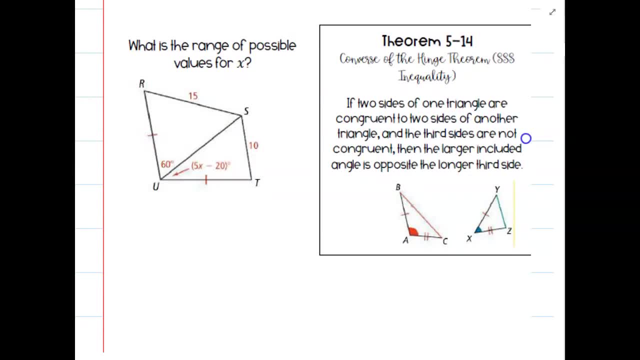 talking about the included angle. okay, now theorem 514 is just a converse of that. so it just says, okay if I have these two triangles. and it kind of relates it. it said, okay if I have these two triangles that have two congruent sides, if this triangle has the 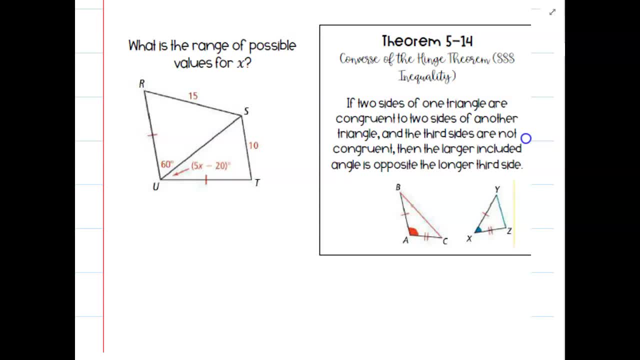 longer side than the other one, this angle is going to be bigger than the other angle on the other triangle. it just is the opposite. okay, so we can use this to kind of like yesterday how we figured out the range of what that third side could be gonna be. kind of like that where what I have here is I have these two triangles. 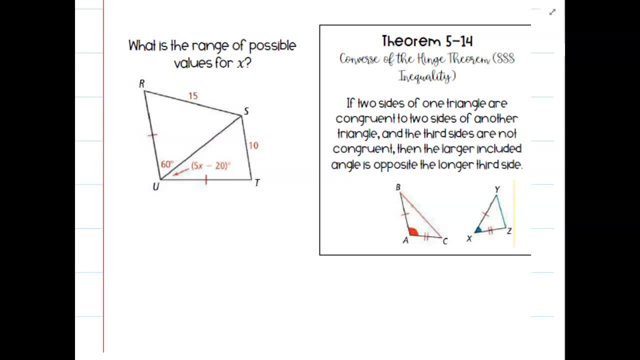 okay, I have two congruent sides. so I have RU is congruent to T. I actually have a second congruent side. I do the reflexive property I have SU be congruent to SU and notice they give me the included angle on both of those. now what I'm looking at is the 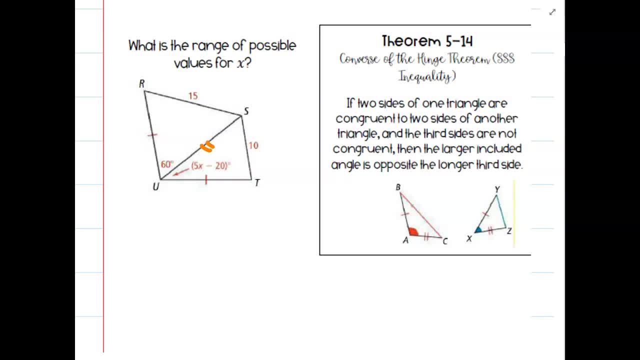 opposite side. so notice, the side opposite of the included angle appears 15. the side off, the side opposite of the included angle is 15 if they're both at the same time on both sides opposite of the included angle here is 10.. So what I conclude here is that what I'm looking for is x. 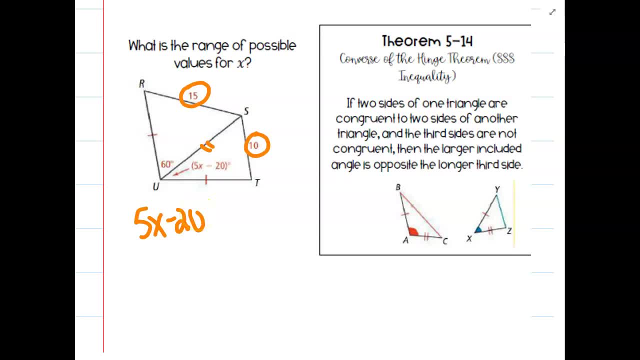 If I start with OK this, 5x minus 20, the side opposite of 5x minus 20 is 10.. So if I wanted to compare that to 60, the side opposite of 60 is 15.. That's bigger. 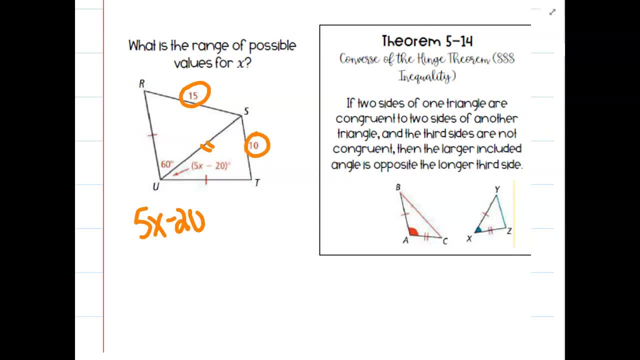 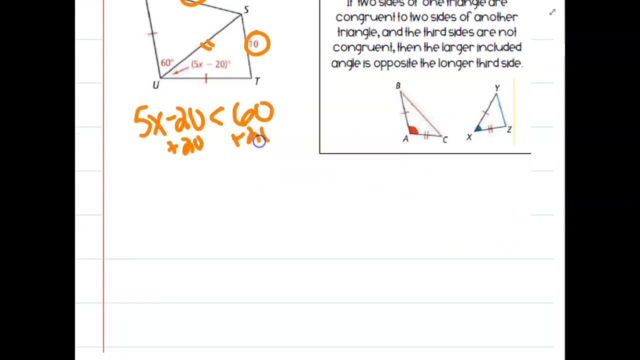 So what it means this is the smaller angle. So 5x minus 20 has to be less than 60. And we can use this to figure out what x could be. So if I add 20, we have 5x is less than 80.. 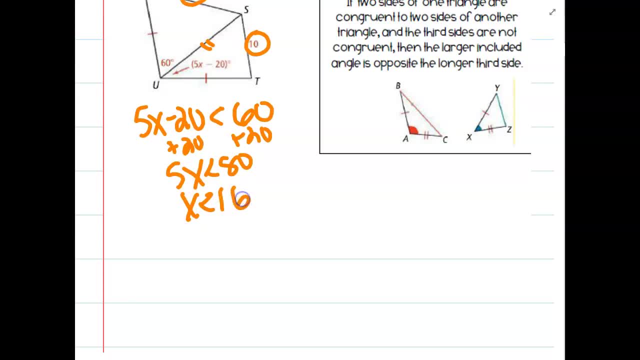 And divide by 5, we have: x is less than 16.. But here's the thing: If I just say x is less than 16, it means that x could be anything less than 16, like 0.. x could be 0, because 0 is less than 16.. 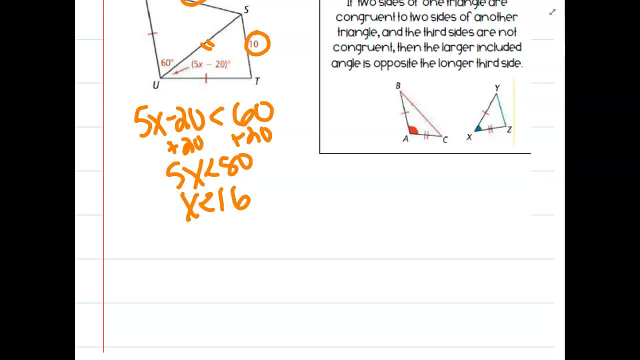 The problem. if I plug in 0,, we have 5 times 0 minus 20,, which is negative 20, which means that angle is negative 20.. Can you have an angle that measures negative 20? No, So you have to figure out the lower limit, right. 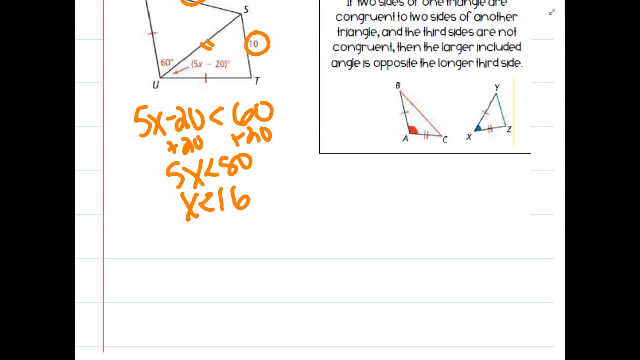 It has to be less than 16.. But I also know that angle that 5x minus 20, 5x minus 20 has to be positive. So 5x minus 20 has to be greater than 0. So then if I add 20, we have 5x is greater than 20,. 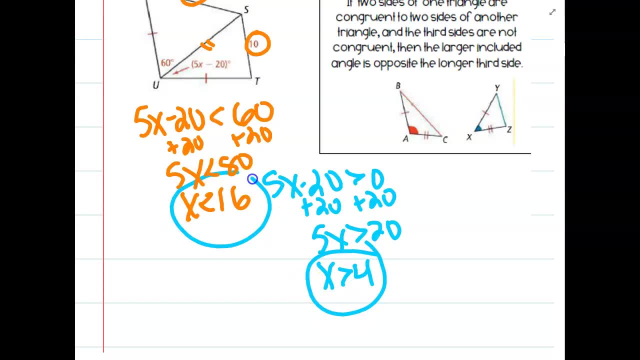 which means x is greater than 4.. So the range for your x values will be between 4 and 6.. That's what we're doing today. That's it, OK. All right, Let's get this glued into your notebook. 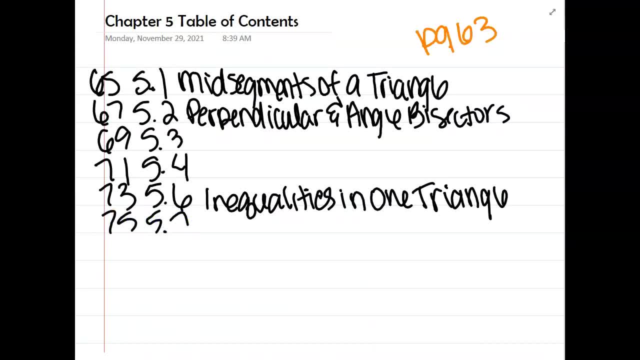 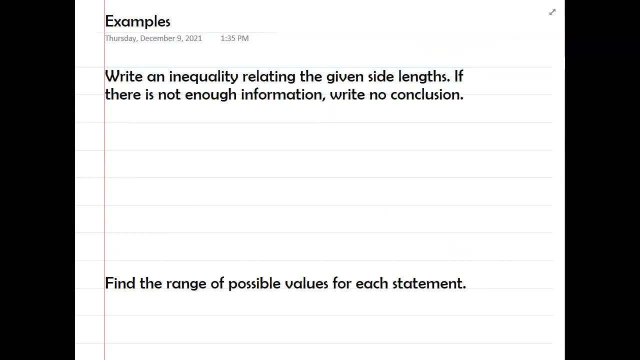 This should be page 75, section 5.7.. And it is inequalities And two triangles on that left-hand side. So mainly two things. So using the Hinge Theorem to relate to side lengths and then using the converse of the Hinge Theorem. 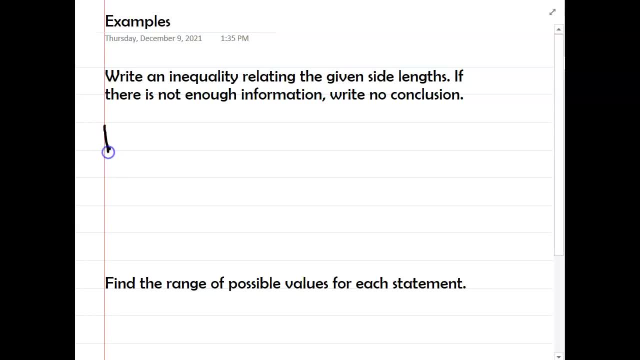 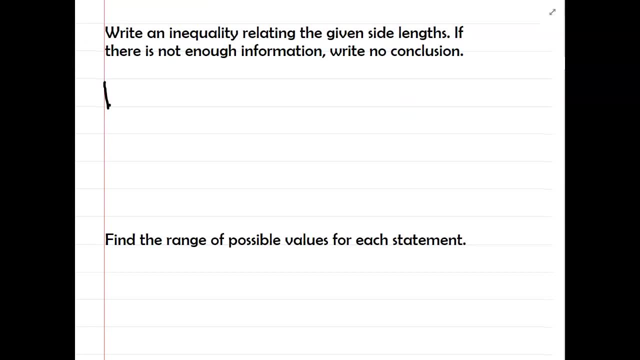 to find a range of values and variables. So we want to write an inequality to relate to a given side length. Now, if there's not enough information, we will just write no conclusion. So, number one, let's draw a right triangle. 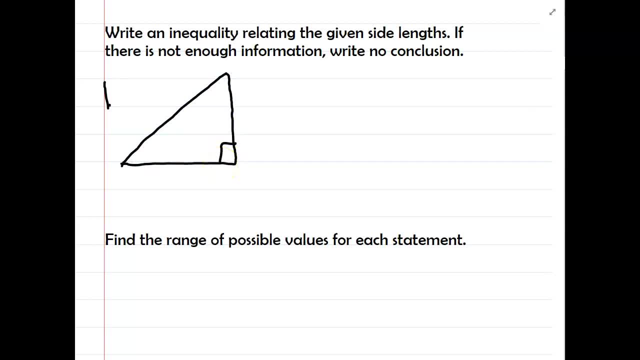 So it will, of course, have a right angle. We'll call this triangle RST, And right next to it let's draw an obtuse triangle like this, And we will call this triangle ABC. Now, to use the Hinge Theorem, you 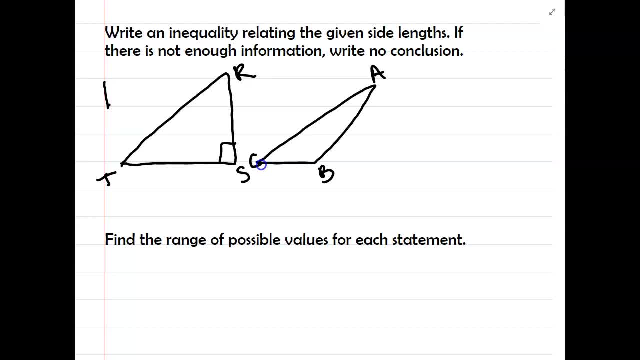 have to have two sets of congruence OK Sides. So we will say RS is congruent to AB, TS is congruent to BC, And then angle B is 98. And finally, we want to write an inequality to relate RT and AC. 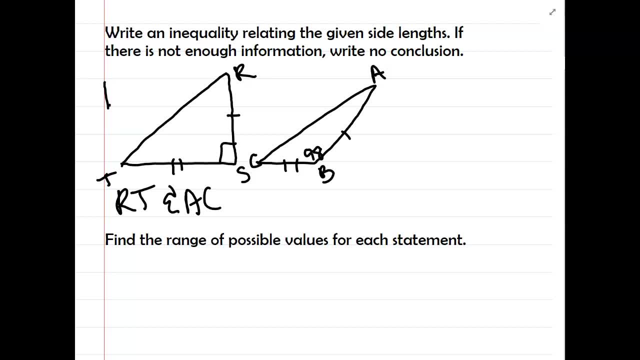 So this is what your homework problems are going to look like. You're going to have the picture And then it's going to say: OK, look at these two side lengths, RT and AC- And I want to state an inequality saying: 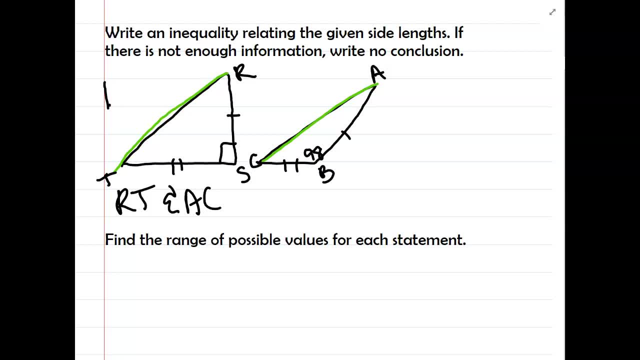 here's what I know about RT and AC. Now, what you need to make sure of: if you're able to use the Hinge Theorem, you have to have two sets of congruent sides, which I do, And you have to have the included angle, which I do. 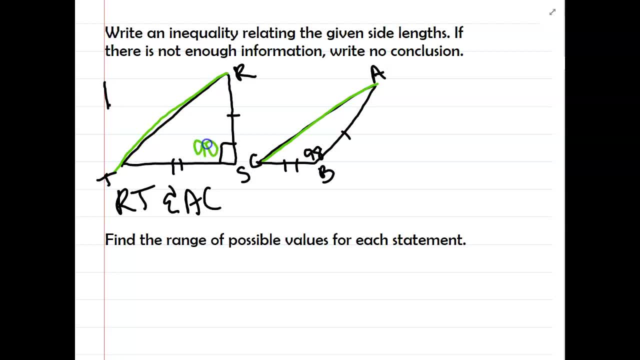 This is 98.. This is 90. 90. 90. 90. Now remember, since that angle is the included angle and since these sides are congruent, the larger angle is going to correspond with the larger side. 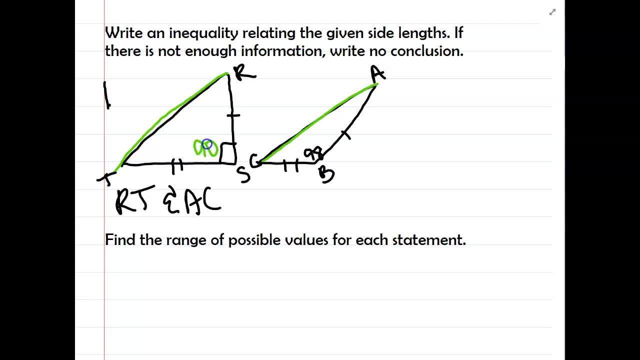 So which is the larger side? Which is the larger side? AC is going to be the larger side. So there's a couple ways you could write your inequality. We could say that RT is smaller than 0, right, So it's less than AC. 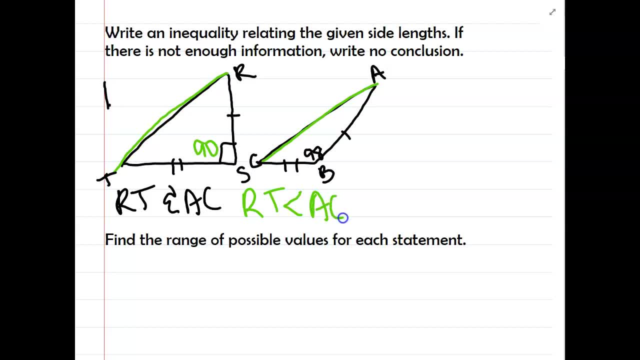 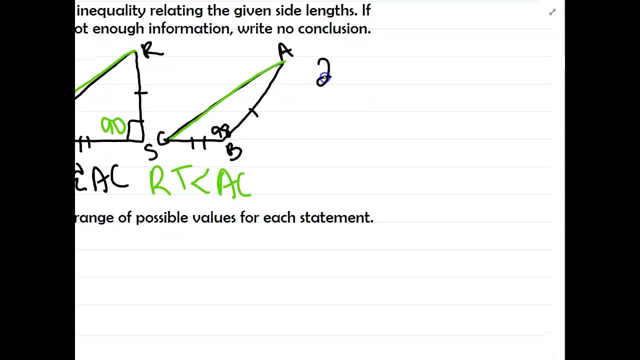 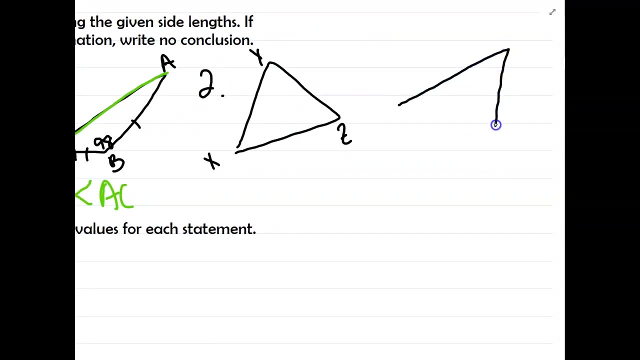 We'll flip them around. We'll say: AC is greater than RT. That's fine, It means the same thing. OK, Number two: Our first triangle is going to be triangle XYZ And the second triangle is going to be ABC. We're going to go XYZ, triangle ABC. 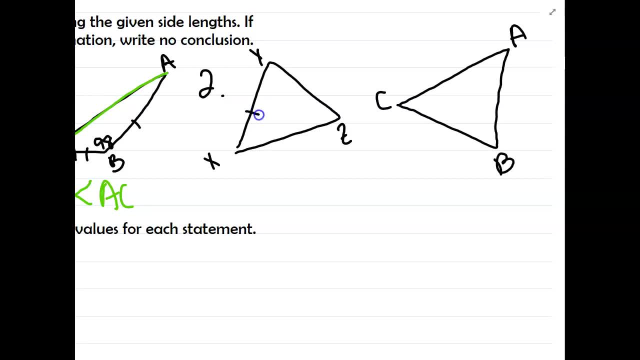 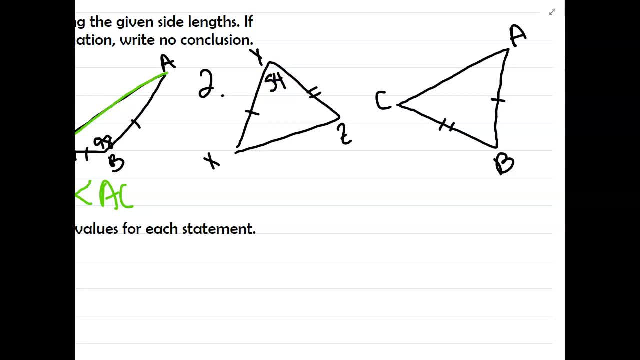 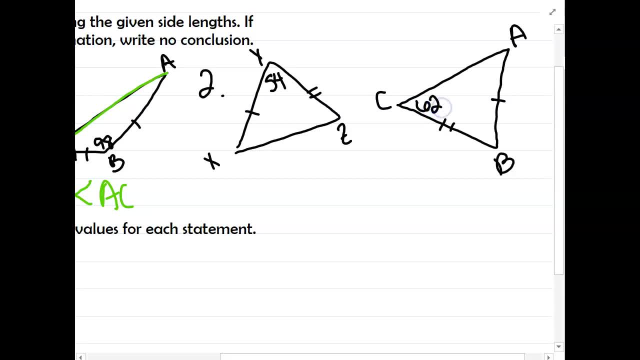 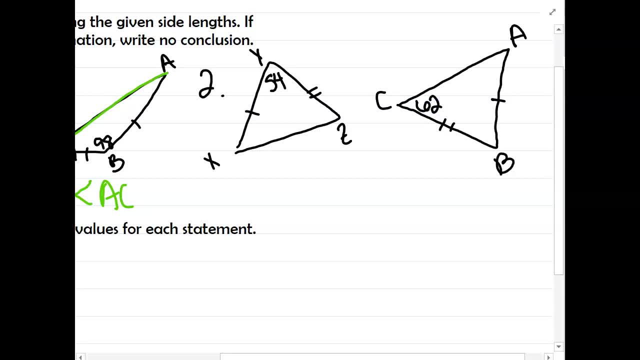 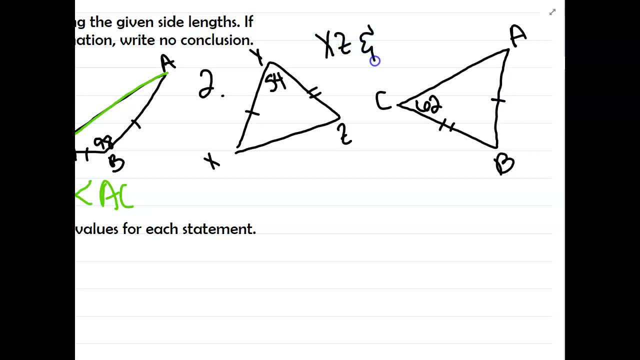 Angle Y is 54.5.. Angle Y is 54.5.. Exactly, Angle Y, it is the included angle right. See how you have the congruent sides, this angle in between them. But here, which angle would you need? You would need this. 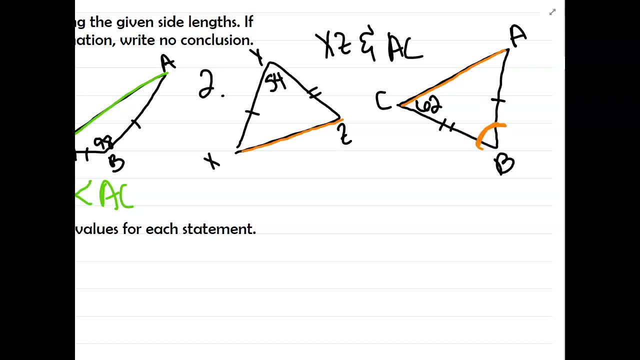 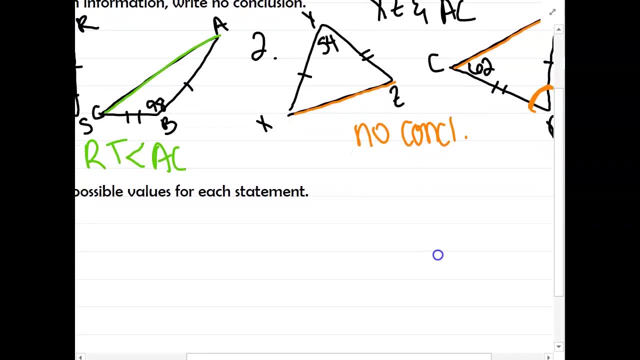 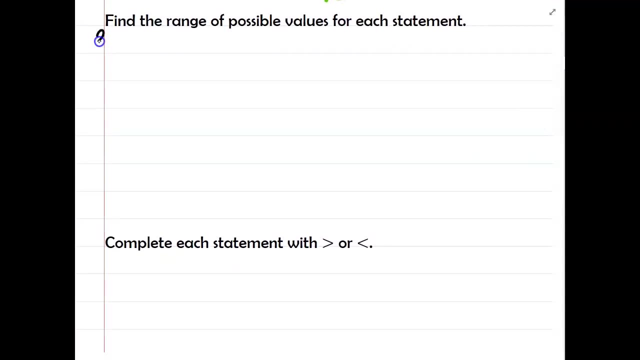 angle right here to do the hinge steering, which I can't, so all you would say is no inclusion. Questions on one or two. Okay, the other ones, we're going to find the range of possible values for each statement. So let's draw a right triangle, our right triangle. 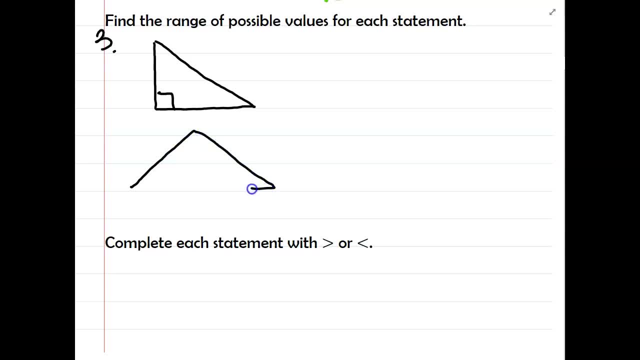 and then a triangle below it like this: Okay, we're going to see, the left side of the right triangle is going to be congruent to the left side, that top left side of the triangle, And then the bottom of the right triangle is going to be congruent to the bottom. 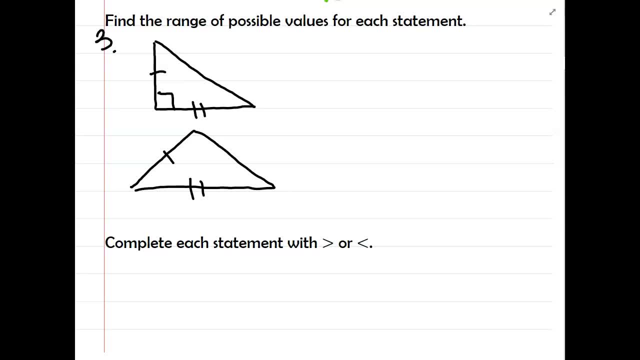 of the other triangle, The hypotenuse of the right triangle, is going to be 15.. And then this side right here is going to be 12.. And then, finally, this angle in the second triangle is going to be 4x minus 8.. 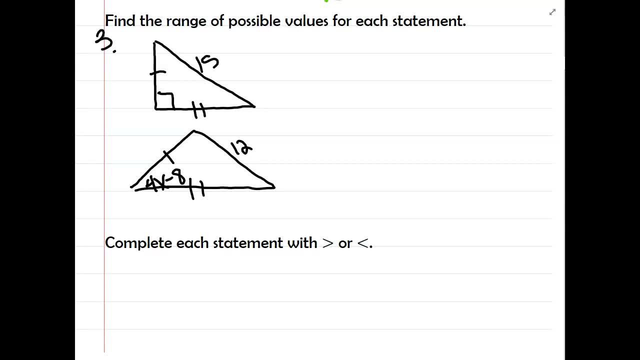 Now I think, typically, what we've gotten really used to is just saying: oh, we're going to set them equal to each other and solve, but I don't know that these are equal. In fact, I probably know that they're not equal, right. But what I do know is I have these. 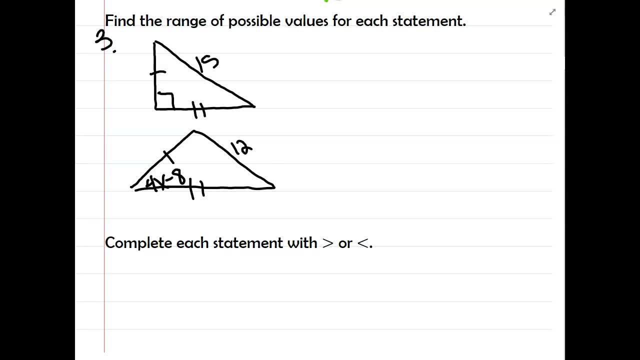 two congruent sides and I have the included angle, okay, And I have the side. I know what the side is opposite of the included angle. So remember, if the side opposite of the included angle, if that's what I have, the bigger angle is the side opposite of the included angle. 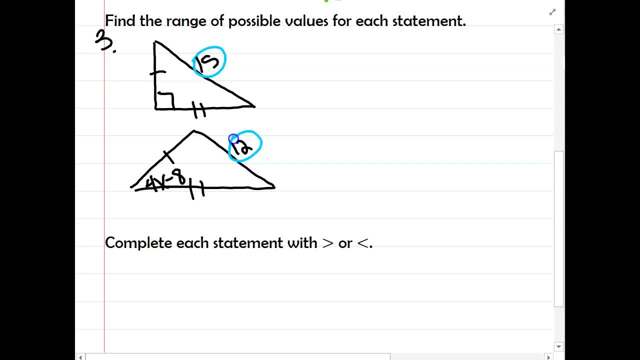 The bigger angle. sorry, the bigger angle is going to correspond with the bigger side. So this right here, that angle is going to be bigger than this one. So if I want to find what x is, I could say: okay, 4x minus 8 is. how would you relate it to 90? It's smaller. 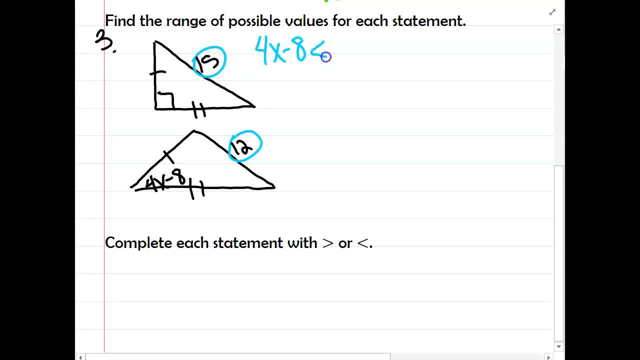 right, Less than because 12 is less than 50. So 4x minus 8 is less than 90. So we will add 8 to both sides We have. 4x is less than 98. Divide by 4, and it gives. 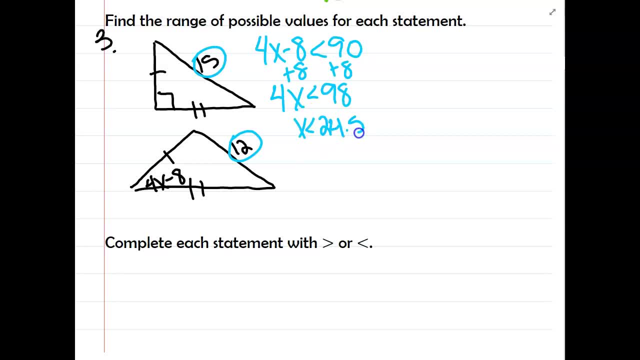 me x is less than 24.5.. Remember, if you say x is less than 24.5, x could be anything less than 24.5, like negative 100. x could not be negative 100. That would give me a negative. 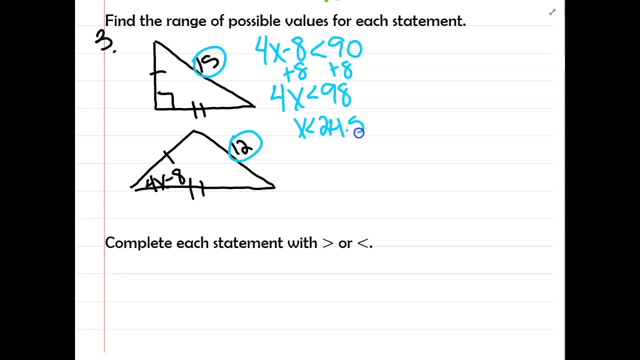 value for an angle, and angles can't be negative. So we also have to say: well, I'm going to say well, whatever 4x minus 8 is, it's got to be bigger than 0,, but it has to be positive. 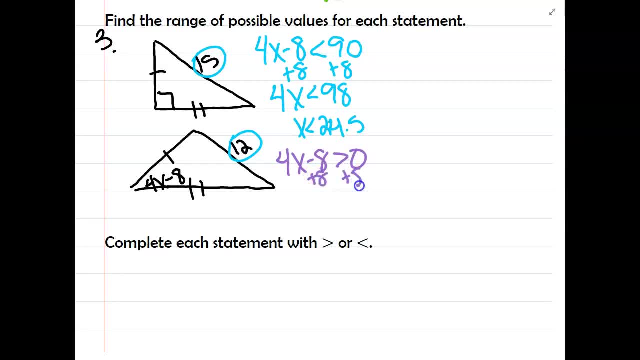 because it's an angle measure. So to solve for x this way, add 8. We would have: 4x is greater than 8. So x is greater than 2.. So x could be any number between 2 and 24.5.. 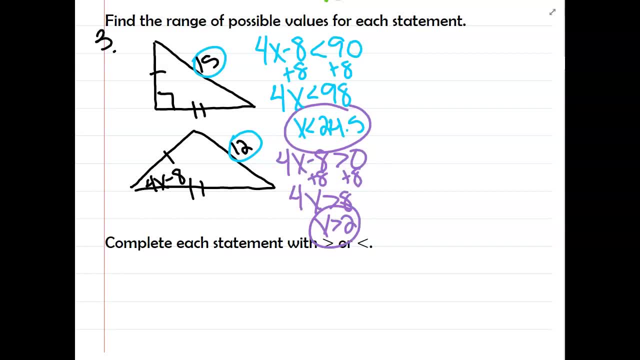 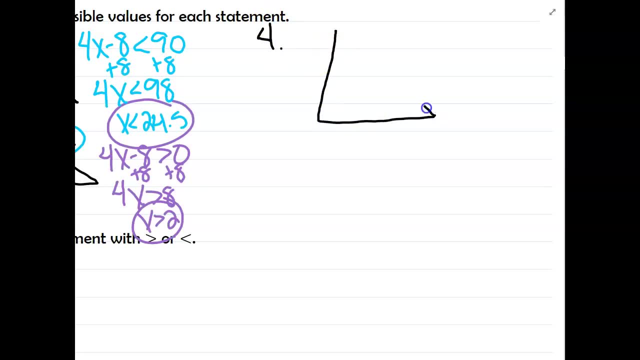 Let's do one more of those, Okay, number 4.. All right, we're going to have this little triangle here, This little triangle here, Okay, and then this left-hand side. let's make that congruent to the left-hand. 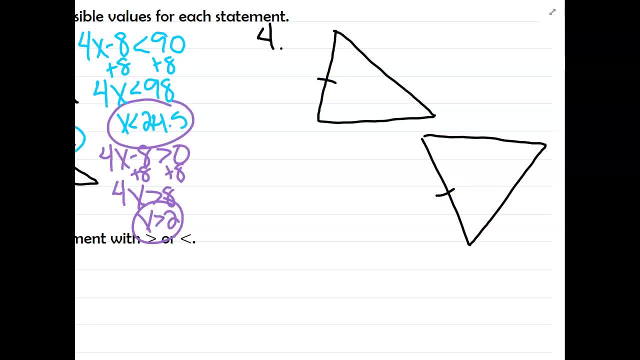 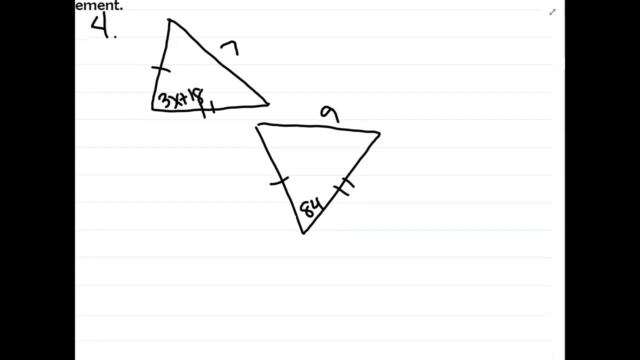 side down here, And then we're going to make the bottom congruent to this left-hand side, This right side. Okay, let's say that that side is 7.. This side is 9.. This angle in here is going to be 3x plus 18.. This angle over here is going to be 84.. So notice if 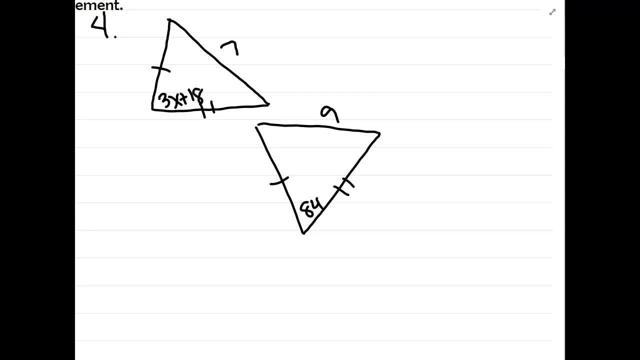 we use the converse of the hinge theorem. we have to have two sets of congruent sides and the included angle and the side opposite, which is exactly what I have. So if I want to solve for x, we say: okay, well, 3x plus 18.. This angle right here, the side opposite. 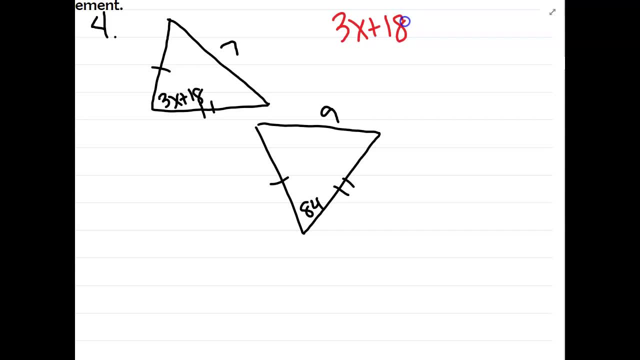 of this angle is 7.. 7 is less than 9.. So 3x plus 18, how would you compare it to 84? It's also going to be less than 84. So we subtract 18 from both sides. 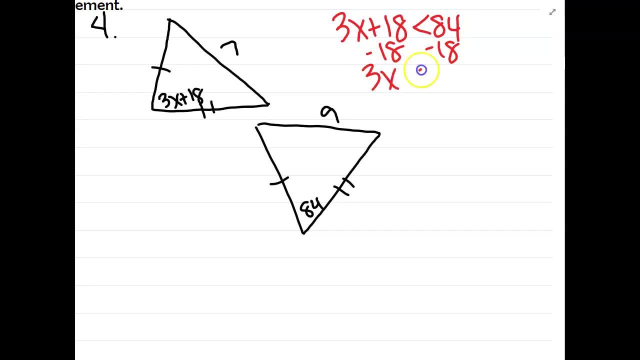 So 3x is less than 66.. So x is less than 22.. What else do I need to find? Yeah, the minimum value, Because I know that 3x plus 18 has to be bigger than 0.. Got one bigger than 0.. 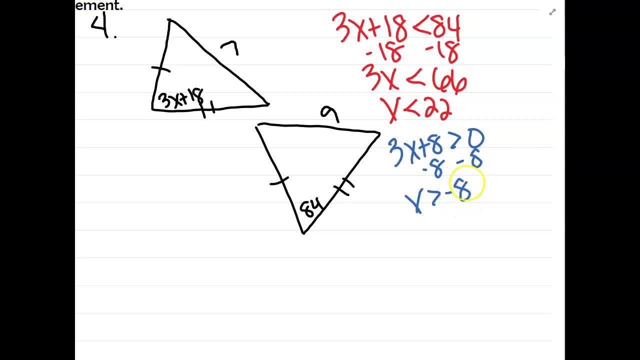 So I subtract 8.. I subtract 6.. 3x plus 18, there we go. 3x is greater than negative 18.. So x is going to be greater than negative 6.. Okay, And then last one. 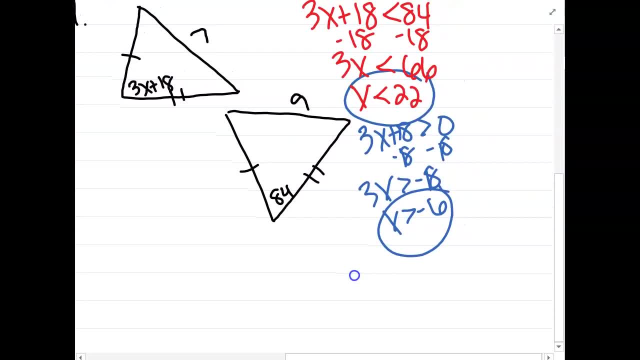 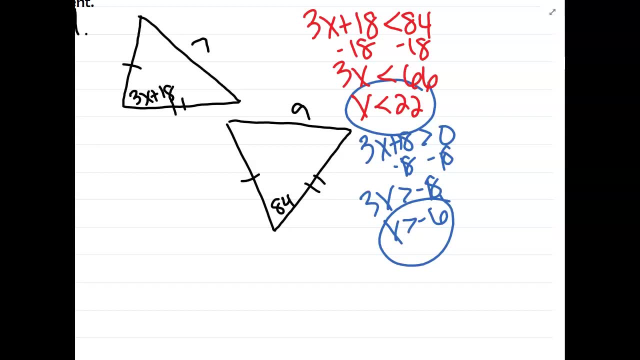 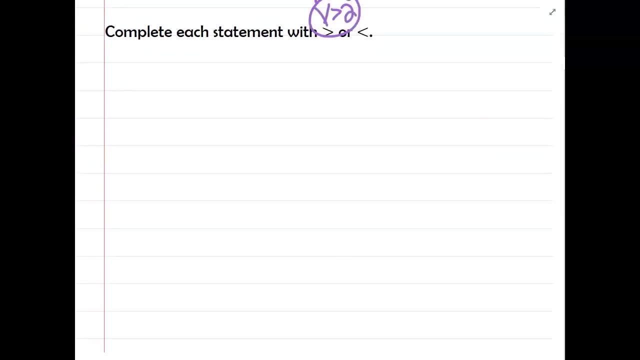 Yes, x can be, Because, notice, even if I plug in negative 1, it would be 3 times negative 1.. It'd be 3 times negative 1, so this can't be negative. Yeah, good question. Okay, last one, and this is going to be a fun little picture to draw. 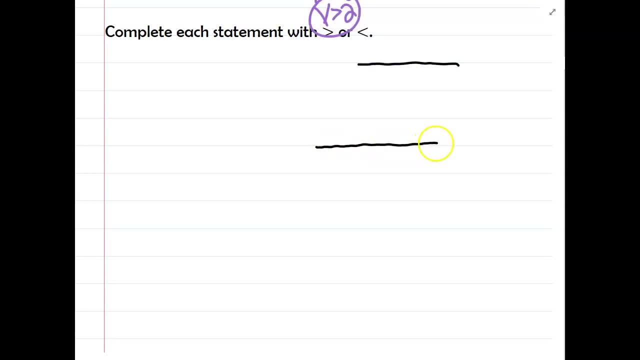 Okay, I want you to draw two parallel lines- The bottom parallel line is a little bit longer than the top one- And then connect them to form a trapezoid Fun word there. And I just told you they're parallel, so let's go ahead and mark them as parallel. 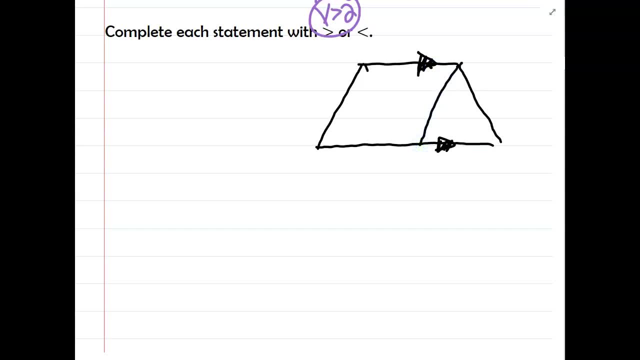 And let's draw triangles here. So we've got kind of three triangles and let's go ahead and label all the vertices. So, starting at the top left and just working our way around, we'll do M, P, Q, O and N. 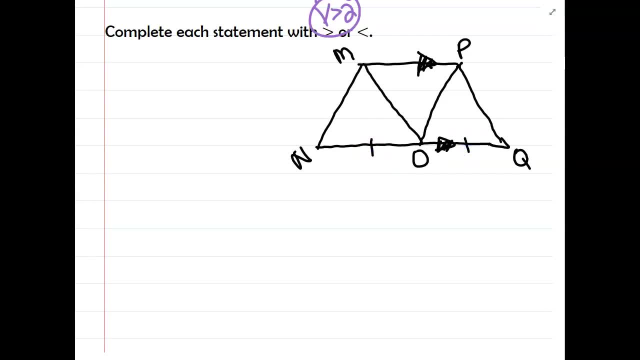 Okay, we're going to say N. O is congruent to O, Q. Both of these top angles here are going to be 45, which means that other angle is going to be 90. And then this angle over here is going to be 44.. 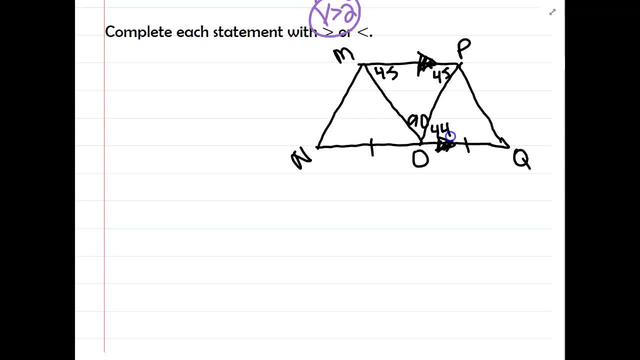 Now, that's all the information I'm given, But I might be able to find some other information Based off this picture. is there anything else that I know, Elijah, So these three angles here together add to be 180. So 90 plus 44, subtract that 180, we would get 46 under that angle. 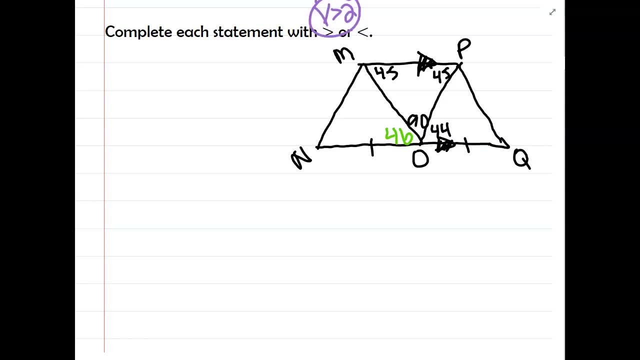 Anything else? Is that maybe enough? Again, N O N. Now, actually they're not See how I have 44, 46? So they're not, And I need to look more at that because I'm kind of weak to do it. 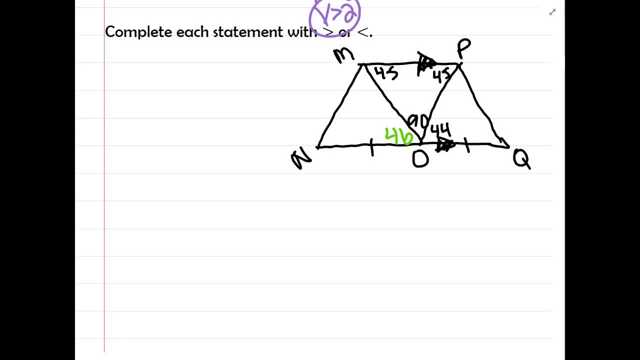 So if we're going to do a parallel line, I think I actually could probably shoot this parallel. What about that middle triangle? What could you know about that middle triangle If these two angles are 45?? It's my sausage triangle. It's my sausage triangle. 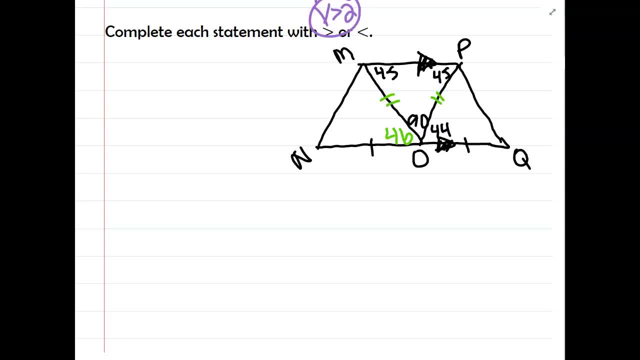 Which means Those two sides are a finger. Okay, So let's use that information. Okay, let's say, if the measure of angle P, O, Q, I want to compare that to the measure of angle M, O, N. 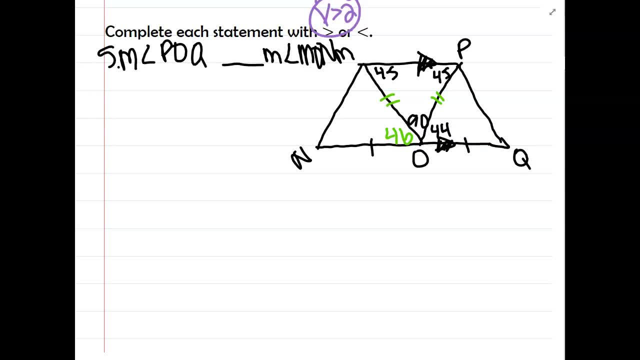 The measure of angle P O Q. The measure of angle P O Q, which they said was 44.. How would you compare that to the measure of angle M O N? Okay, number six, Using that information: M N. how would you compare that to P Q M N. 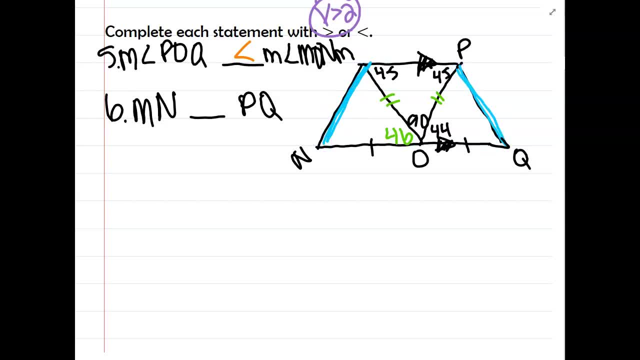 How would you compare that to P Q? It has to be right, because this is a bigger angle. They have two sets of congruent sides, So the bigger angle is going to be opposite the bigger side. And last one, What about M P? 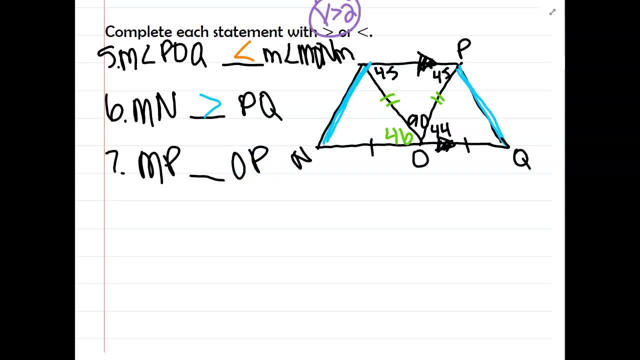 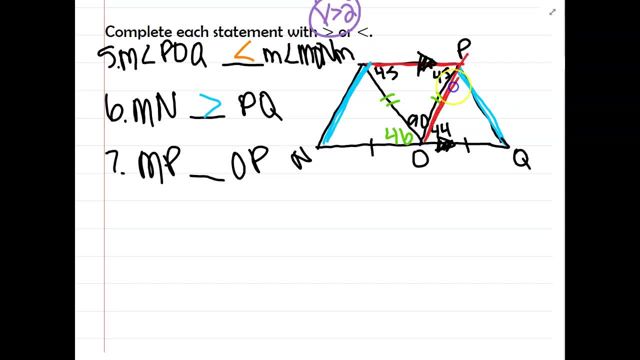 How would you compare that to O P? I agree with that. M P is greater than O P. but how do you know that? Yeah, Remember yesterday we talked about inequalities. in one part, the larger angle- 90, is bigger than 45,, which means that side is going to be bigger than that side.